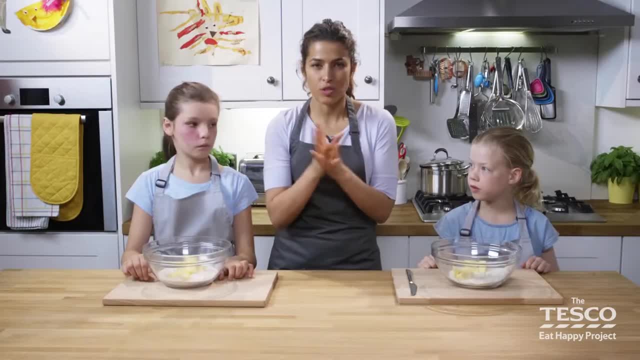 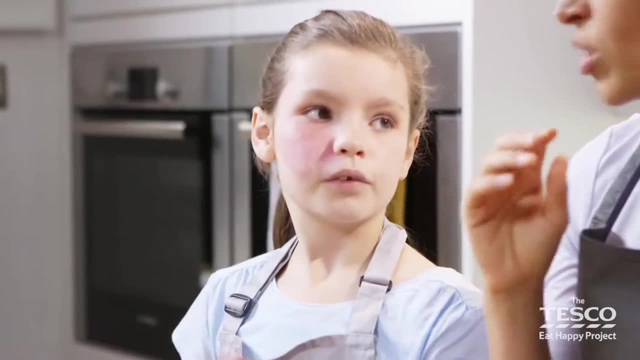 already and I'm going to give you a little tip with your fingers. If you rub your hands together very quickly and put your palms on your face and then on your fingertips, Which bits are the hottest bits and which ones are the colder parts? Colder are your fingertips and the hotter are your palms. 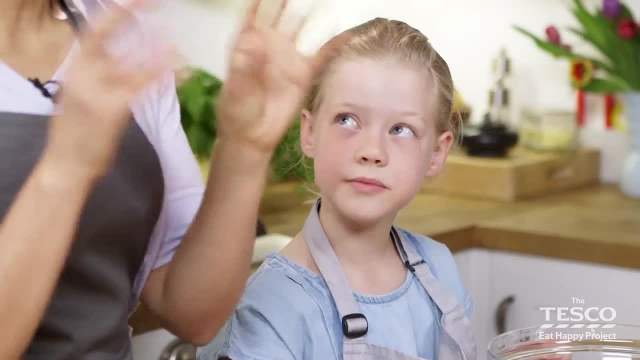 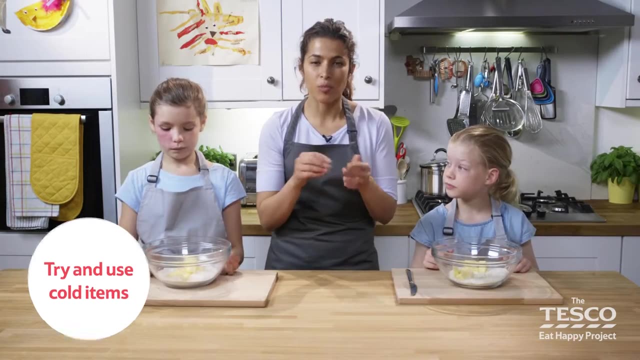 Brilliant, well done. So to not let the butter melt, we need to use our fingertips. We need to use cold fingers, cold butter, cold bowls. This helps it rub in really well and to make them almost like breadcrumbs. If it's too warm then they'll go too smooth. So, girls, what I'm going? 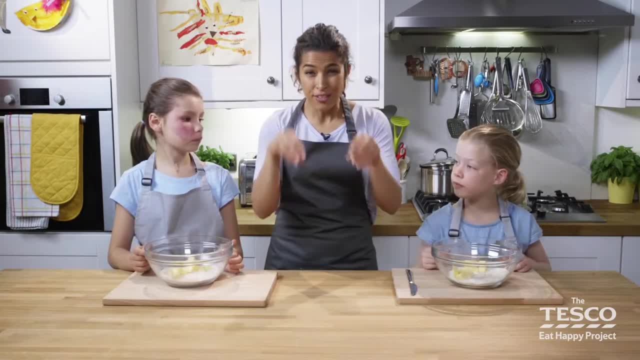 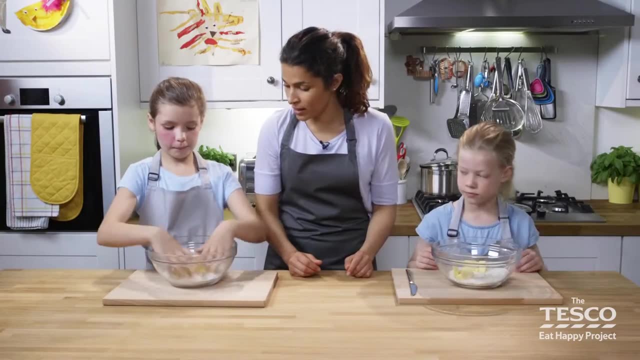 to ask you to do is use your fingertips only to lift up the pieces of butter and give them a little squeeze at the top, and then drop them back down and keep going Ready. Go on, then give it a whirl for me, just your fingers, You'll notice. 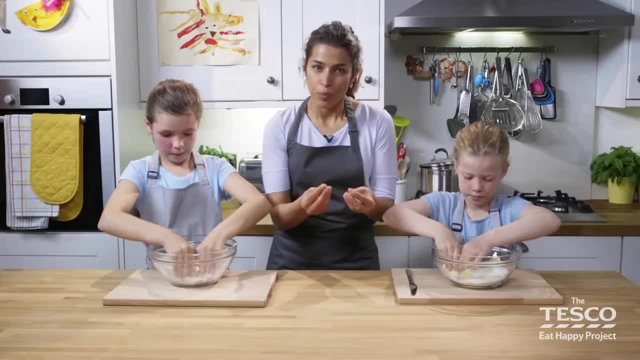 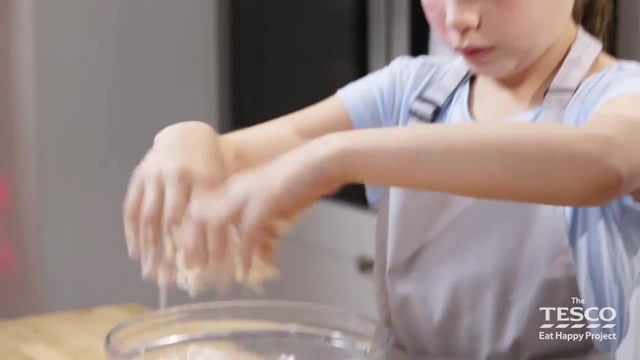 then that you won't have the flour on the palm of your hands. If you do, don't worry, but what we need to use are these fingertips. Well done, Lola. Can you lift it a little higher so all the children can see, and give it a little squeeze and drop Madelena? brilliant. So, Lola, what does it feel like? 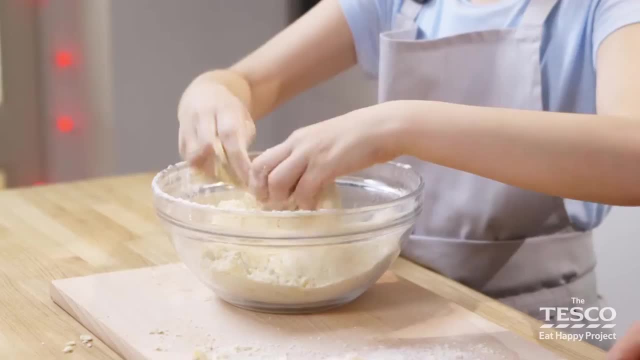 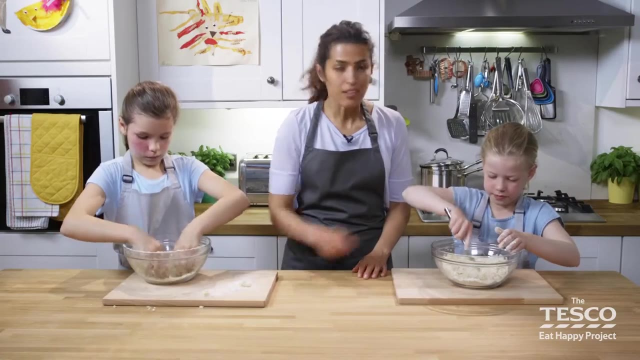 It feels quite now. afterwards it feels quite crumbly. Oh, it looks fantastic. you two, Do you want to have a go with the knife? Madelena? Where's your knife? So that's the way of cutting through with a knife, and it brings it all together eventually at 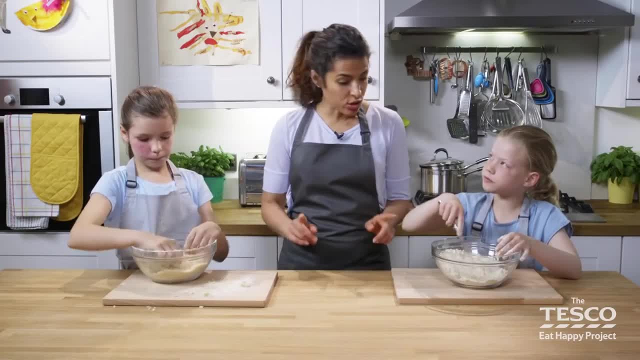 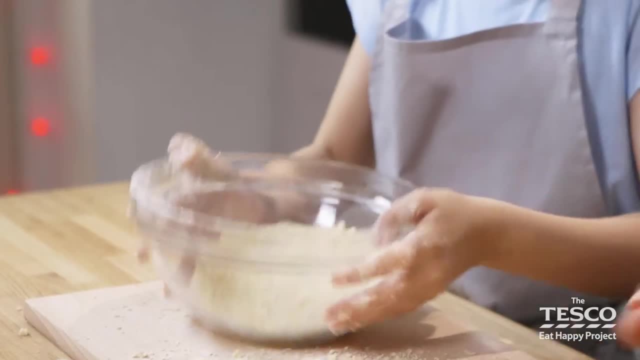 the end. Good work, Madelena. So, girls, a really good top tip is to grab hold of the bowl, give it a little shimmy. There we go and a shake and it lifts up all the big bits to the top and allows you to make them smaller again. Lola, I think you're done. That is fantastic. Look at that. 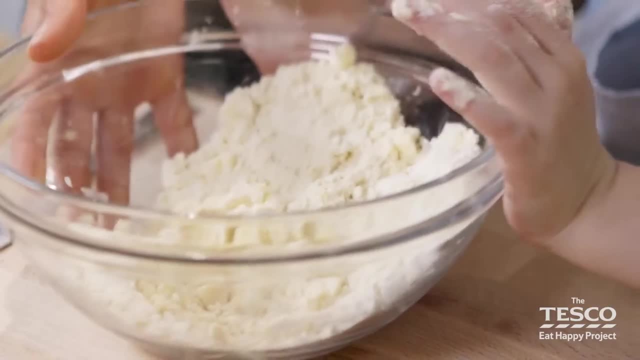 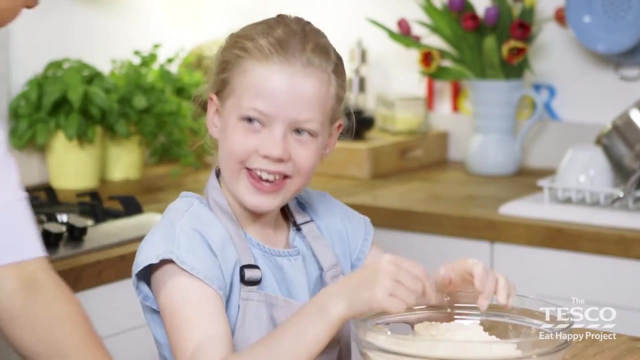 There we go. Madelena, that's wonderful, Brilliant work. Do you want to rub off your hands over the bowl? girls? Get all the rest off. That's it Well done. Did you have fun doing that, Madelena? Yeah, Did you Lola? Yeah, I hope. you had as much fun too. Bye.